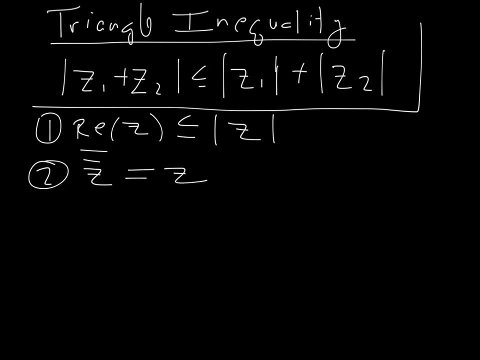 conjugate twice, I get back to my original complex number. And these are pretty simple. The first one proved in class and the second one is one of your homework assignments. So with that stuff in mind, let's go ahead and look at how the proof is going to work. So, 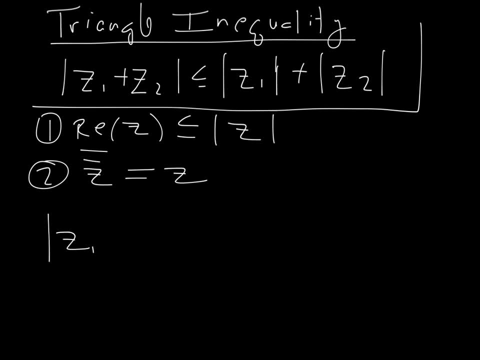 we'll start out by looking at the absolute value of z1 plus z2.. So we'll start out by looking at the absolute value of z1 plus z2 squared. So in class we saw that this is just z1 plus z2 times z1 plus z2 conjugate. Now, if it's a property of conjugates, this: 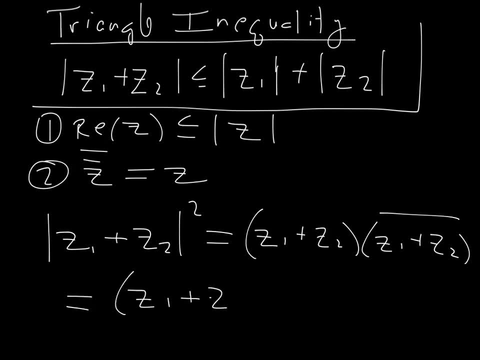 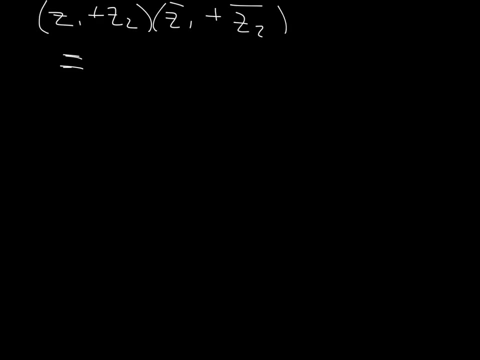 is just equal to z1 plus z2 times z2 squared Now, if we look at the real part of any complex times, the conjugate of z1 plus the conjugate of z2.. So if we go ahead and multiply this out, we're going to get z1, z1 conjugate plus z1, z2 conjugate. 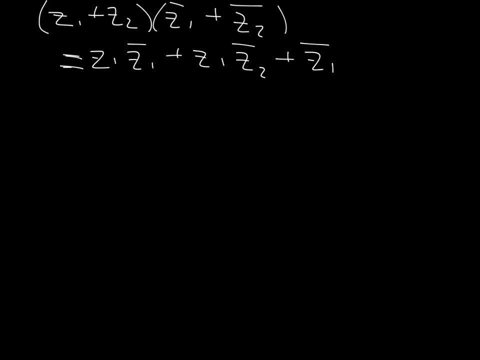 plus z1 conjugate, z2 plus z2, z2 conjugate. So this is the absolute value of z1 squared plus z1, z2 conjugate plus. Now notice what I'm going to do here. This is z1.. 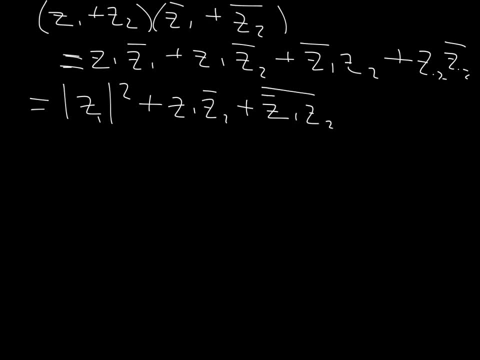 z2.. But I'm going to do the conjugate over that twice And we'll come back to that in the next line, And then plus the absolute value of z2 squared. So this is the absolute value of z1 squared plus z1, z2 conjugate plus. 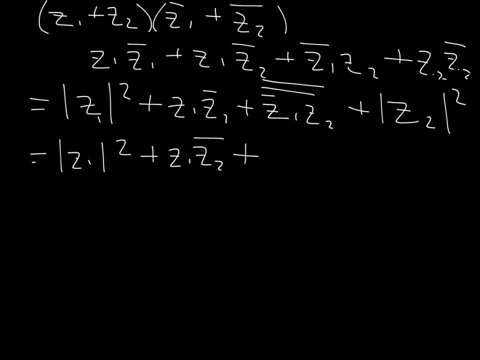 Now by taking the conjugate twice in this one. notice what happens. I'm going to get z1, z2 conjugate from applying this first one, These first two rather, And it's going to be the conjugate of that. 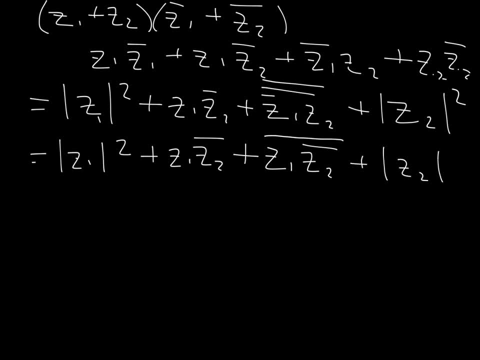 So then, plus the absolute value of z2 squared. Now this term right here is one of our expressions for the real part of z1 times z2 conjugate. So this is going to be equal to z1 squared plus 2 times the real part. 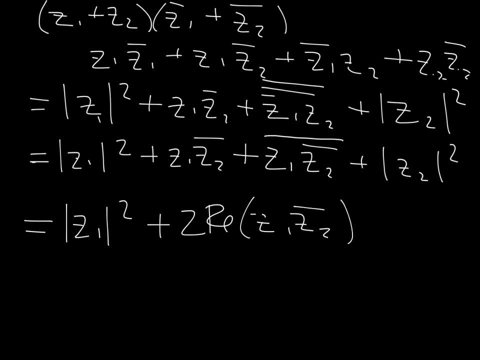 So this is going to be the conjugate of z1, z2 conjugate plus the absolute value of z2 squared. Now I'm going to use the first of those facts I talked about And note that this is less than or equal to. 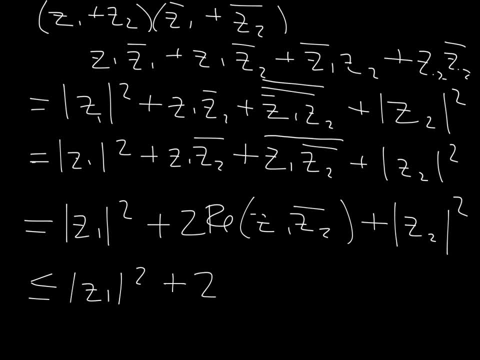 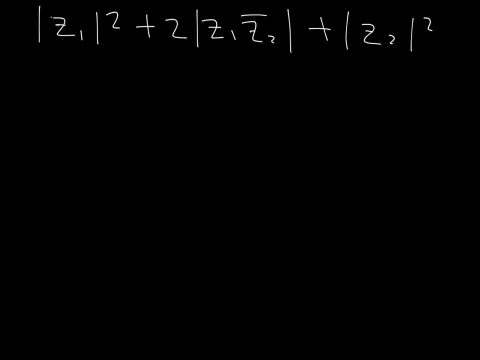 the absolute value of z1 squared plus 2 times the absolute value of z1, z2 conjugate plus the absolute value of z1, z2 conjugate. So this is equal to z1 squared. Oops, let me try that again. 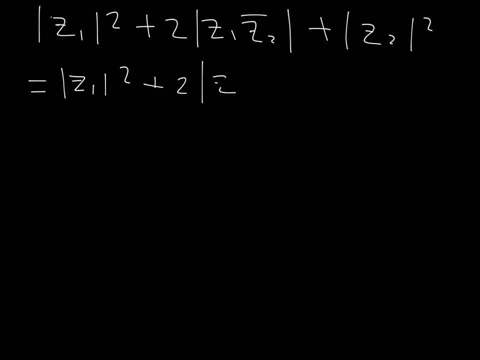 z1 squared plus 2 times the absolute value of z1, times the absolute value of z2 conjugate plus plus the absolute value of z2 squared. But it's one of the properties of conjugates: The absolute value of the conjugate. 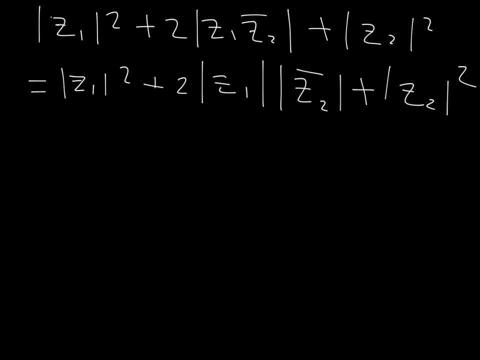 is the absolute value of the complex number. So this is z1 squared plus 2 times absolute z1 times absolute z2 plus z2, or absolute squared. But now this will factor into absolute z1 plus absolute z2, quantity squared.